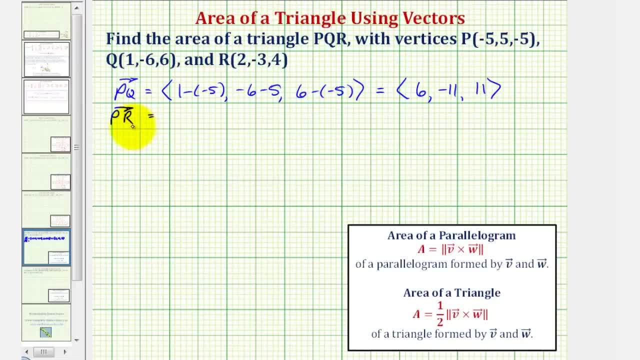 of positive eleven. And now for vector PR. the x component would be two minus negative five. the y component would be negative three minus five. the z component would be four minus negative five. So vector PR has an x component of seven, a y component of negative eight and a z component. 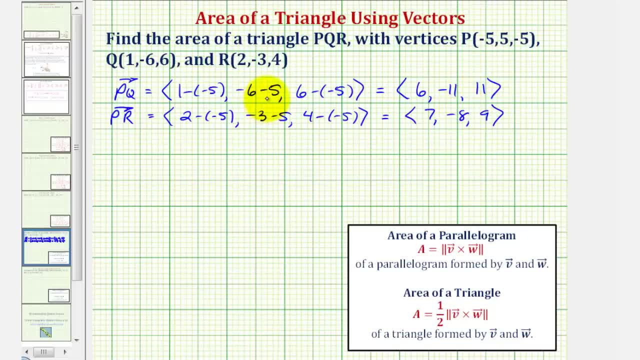 of positive nine. Now that we have the two vectors that form the triangle, we'll find their cross product, And we'll do this using a three by three determinant. So the first row will be the unit vectors i, i, j and k. 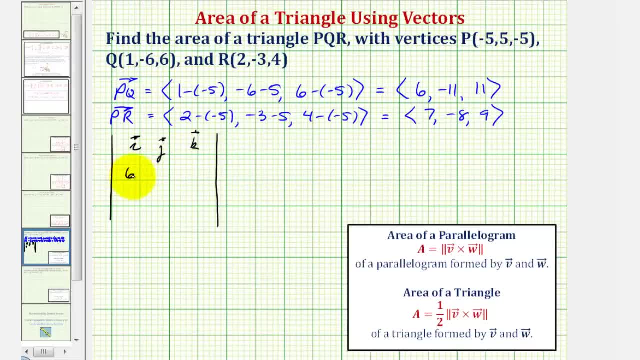 The second row will use the components of vector p- q, so we have six negative 11, 11.. The third row will be the components of vector p- r, so we'll have seven negative, eight and nine. This will be equal to a two by two determinant. 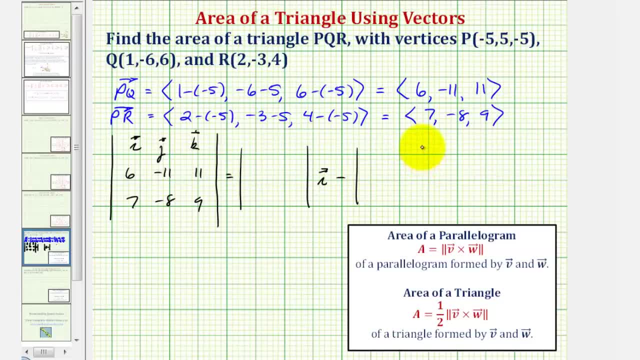 times the unit vector i minus a two by two determinant times vector j minus a two by two determinant times vector k. And now to find the elements in this first two by two determinant, we'll eliminate the row and column of vector i. 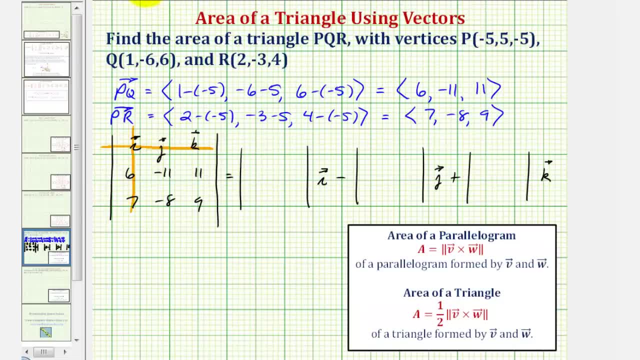 so we eliminate row one, column one. The remaining elements are the elements in this first determinant. So we have negative 11, 11, negative eight and nine. Next we'll eliminate the row and column of the unit, vector j. so we'll eliminate row one again. 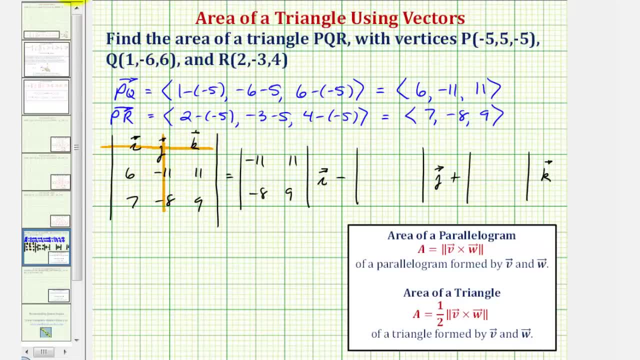 and we'll now eliminate column two. So the remaining elements will be six, 11,, seven and nine, And then, for this last determinant, we eliminate the row and column of unit vector k. So we eliminate row one again, but now we eliminate column three. 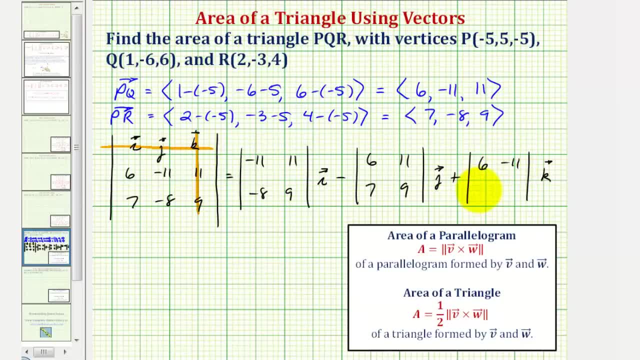 So this would give us six negative 11,, seven and negative eight. And now we'll write this first determinant Here we'll have negative 99, and negative eight, So we have 99 minus negative 88, which becomes negative 99 plus 88.. 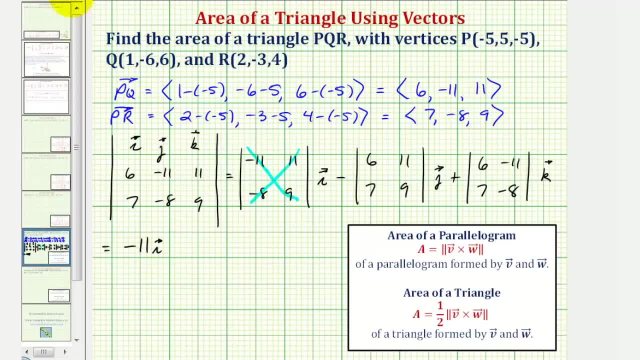 So we have negative 11i Here, we'll have minus, and then 54 minus 77,, which is negative 23.. So we have minus negative 23,, which becomes plus 23j, And then, finally, we have plus negative 48.